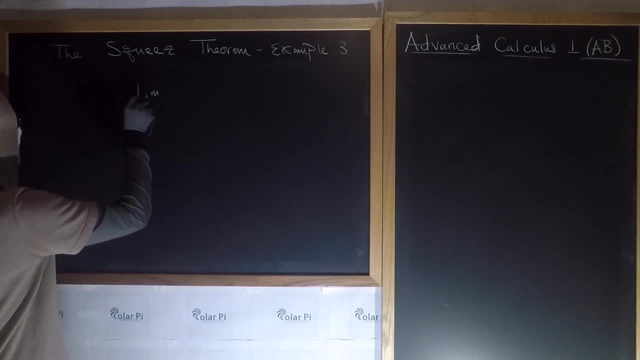 three. In this example we're going to look at this limit. Limb is n goes to infinity, of seven to the n over n, factorial. Yeah, Okay, Now you don't have to use a squeeze theorem to prove this limit or to show what it is, But here, of course, we're using the squeeze theorem, So we 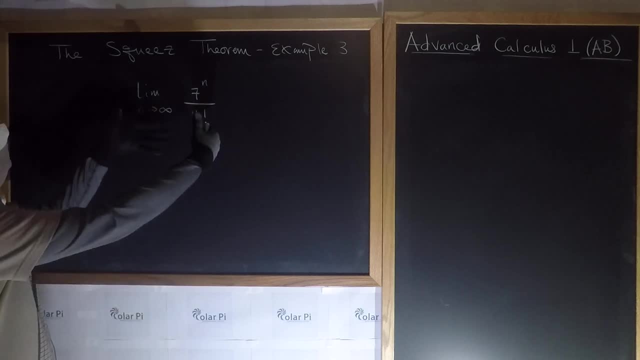 need to figure out how to squeeze this seven to the n over n factorial. But however you think about this, you cannot depart from the following line of thinking, which is like: seven to the n right, Seven to the n Is n sevens in a product, So that's like seven times seven times seven. I'm not going to write. 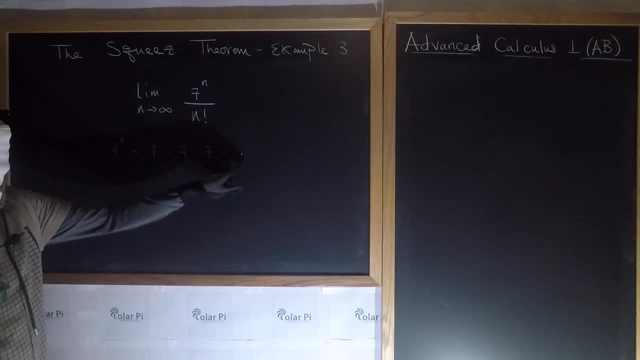 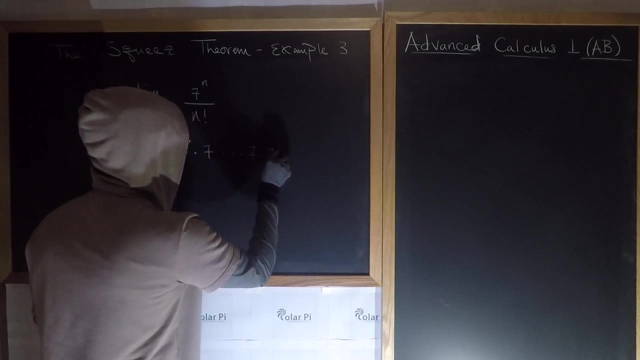 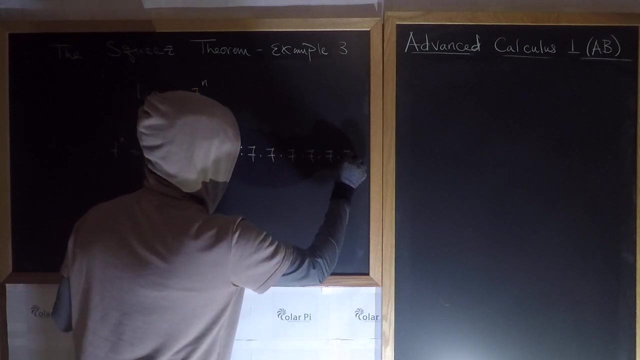 too many sevens, Don't worry, But I will intentionally write seven sevens after this, because it will help a lot of you understand this. Yeah, So seven times seven times seven. four, five, six, seven. So I've got seven sevens here. 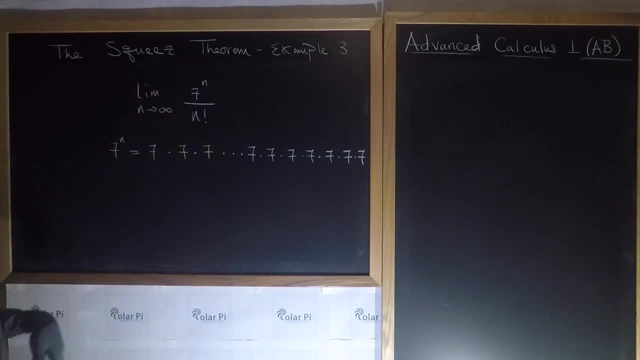 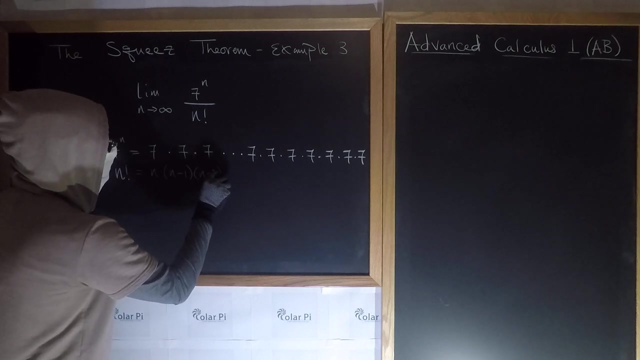 And three sevens here and a bunch of sevens in between to make n sevens right, That's what seven to the n is And n? factorial. we've been through this before. But yeah, n factorial is equal to n times n minus one. All right, Dot, dot dot. What's the tail end of n? factorial? 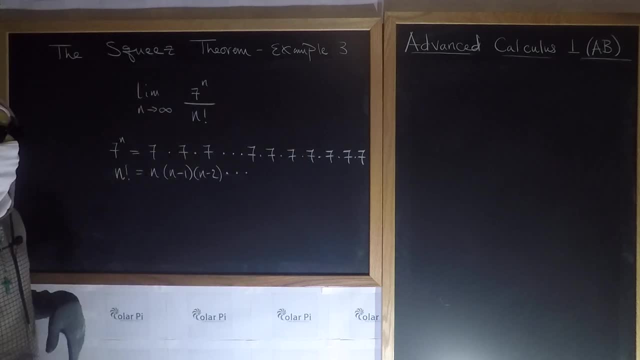 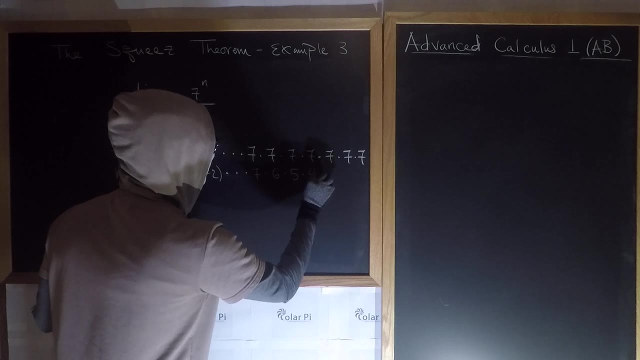 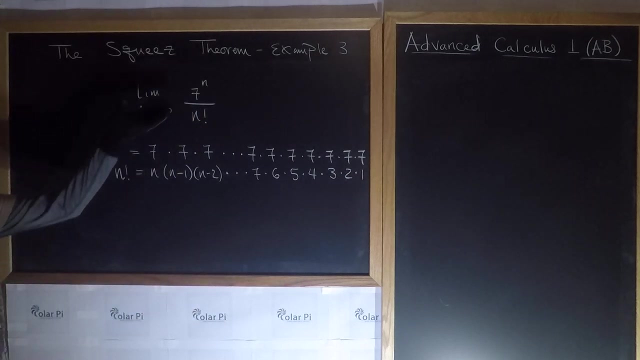 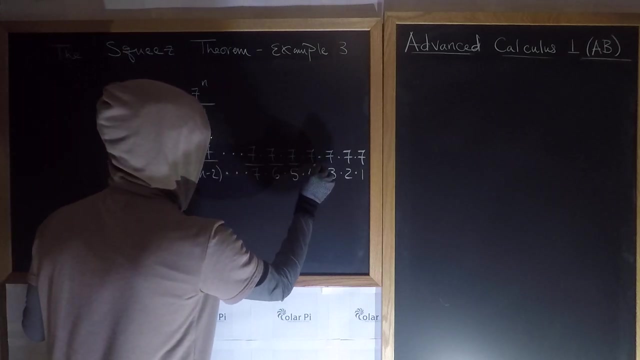 going to be, In fact, the last seven in n factorial. they're going to be seven times six times five, right, Okay? Now, since we have a quotient here, I need to put a division sign here And, as we've already said in previous examples, I could put individual division. 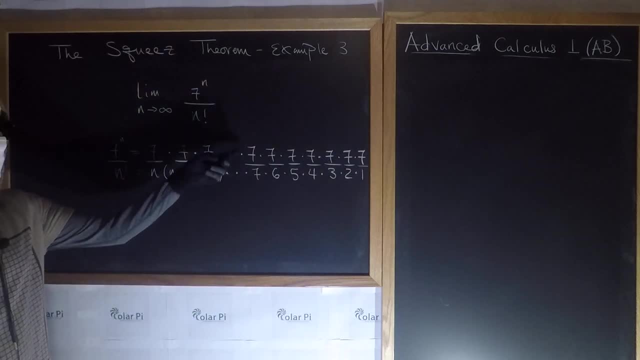 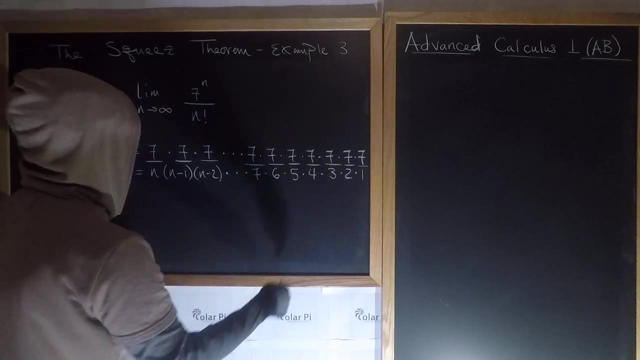 signs here. Now notice clearly: seven over seven is one, But all the fractions in here are more than one. Seven over six, all the way to seven over one, There are more than one. So to make n factorial, we're going to have n factorial. So we're going to have n factorial. 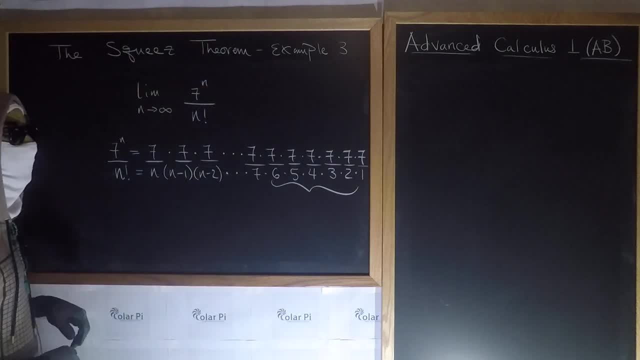 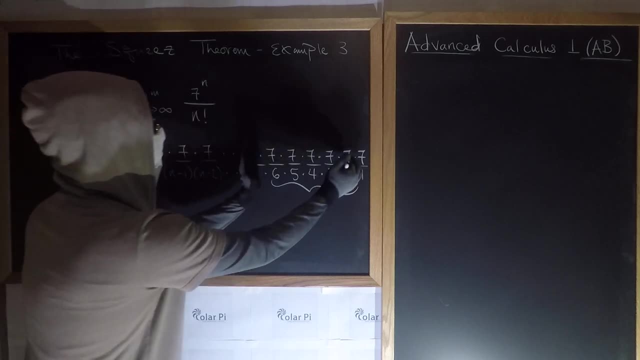 here. So if we want to keep the analysis simple, let's keep these guys, And so that's to say that let's work with this and figure out how to bound this without tampering with this right Now. how can we succinctly write this? It's seven to the six over six factorial. 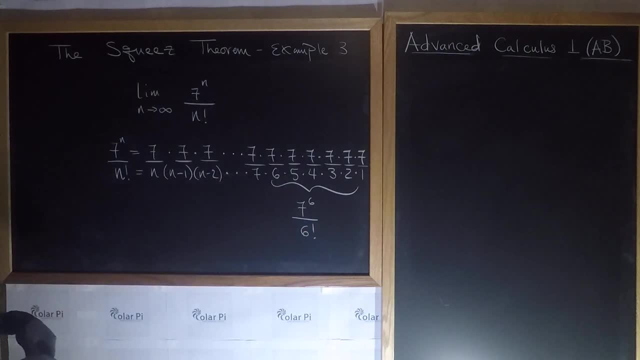 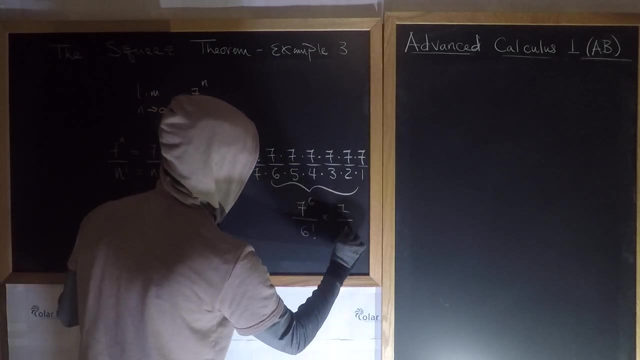 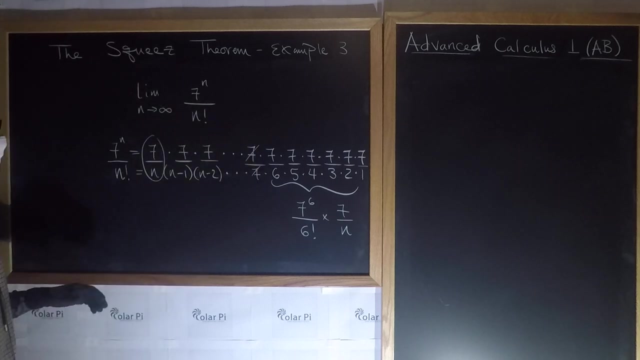 right, That's what I've underlined here. It's seven to the six over six factorial. Let's also keep seven over n, So I have times seven over n. Yeah, Okay, So I've kept this, I'm going to keep this And I've kept all of these guys. This is clearly one right, But all. 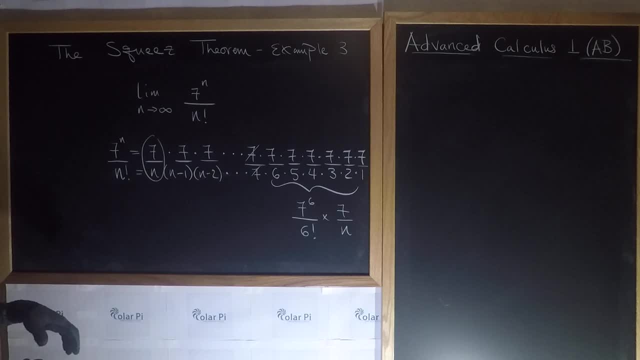 of the fractions in here right, And how many of them is there? There's n minus eight fractions. All of these guys. they're all less than one Because, like immediately to the left of seven over seven is going to be seven over eight, which is less than one. And immediately to 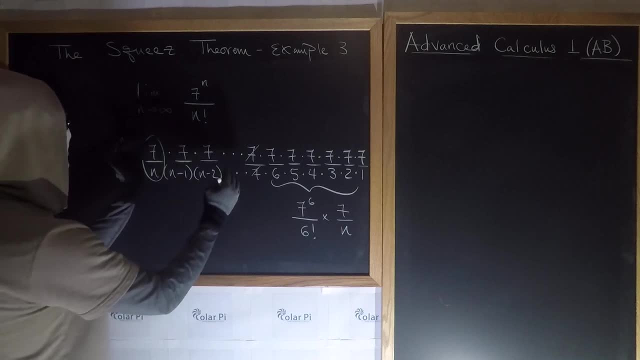 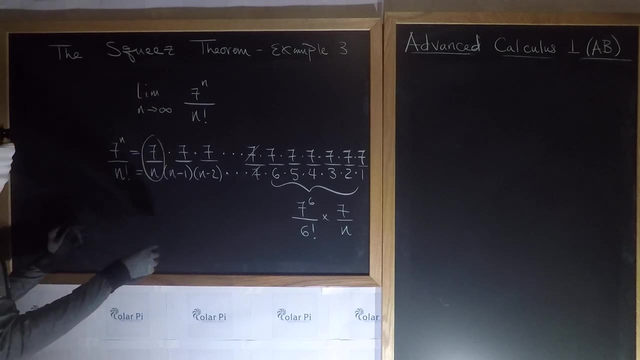 the left of it is going to be seven over nine, which is also less than one. So the n minus eight fractions in here are all less than one. So if we replace all of them by one we're going to get one. Then surely I can say this: which is seven to the n over n factorial is. 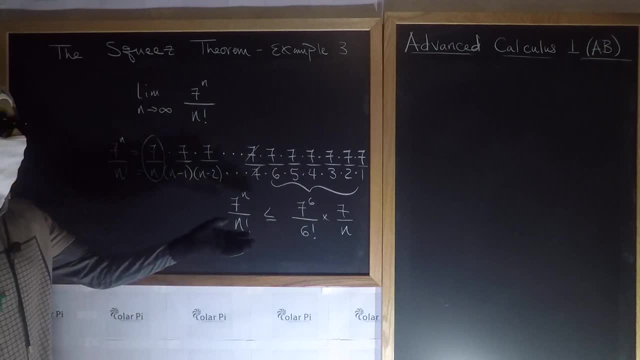 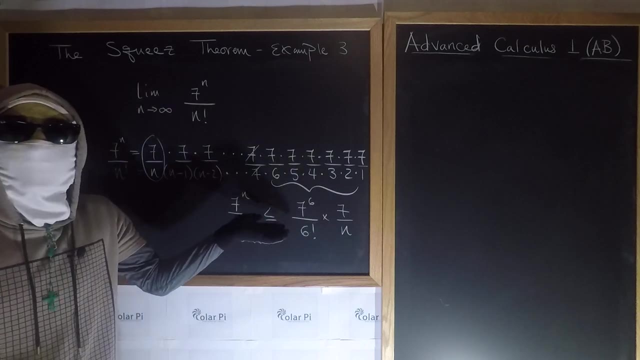 less or equal to this. Why? Because what I've done is I've taken the n minus eight fractions in here and I've replaced them all by one on this right hand side, And of course I don't want to write one times, one n minus eight times. I could just leave it alone, right? 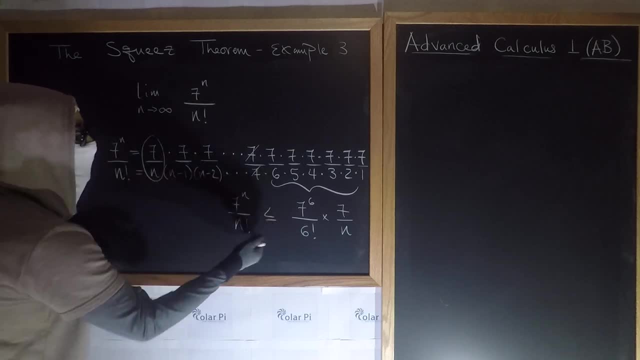 Whereas this guy here contains these guys that are less than one, And that's why this inequality is true. We've now succeeded in finding one way to squeeze seven to the n over n factorial, at least on the right side, And so let's write that result here, So we see that seven to 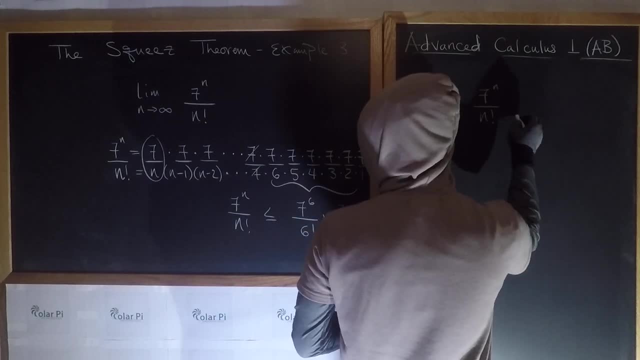 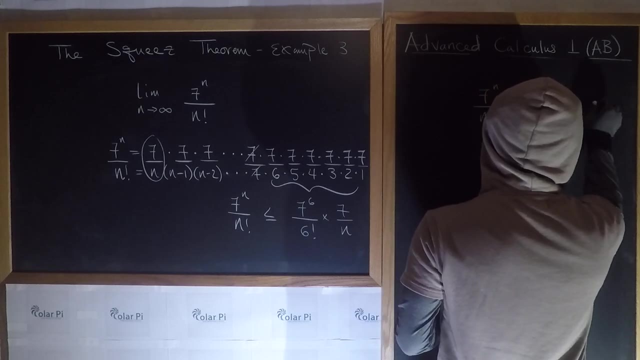 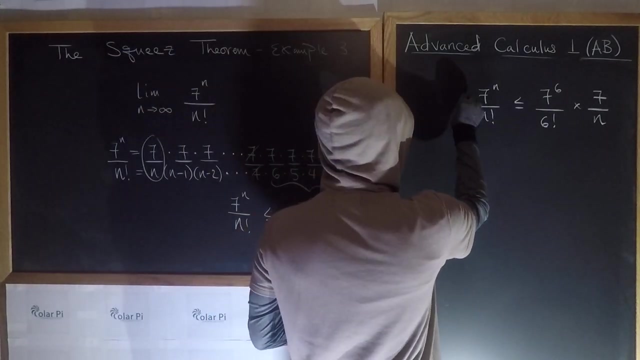 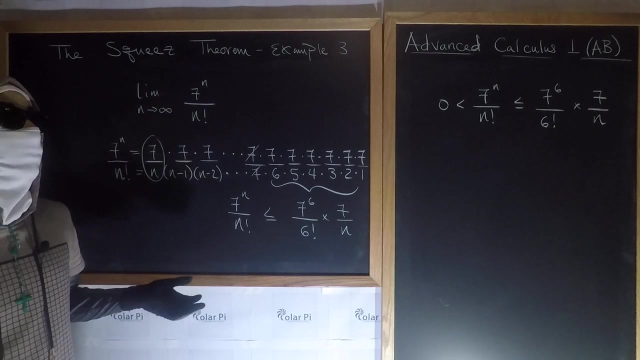 the n over n factorial on the right side can be squeezed by seven to the six over six factorial times seven over n right, And on the left, seven to the n over n factorial is clearly more than zero. So on the left I could write that: Yeah, Okay. So now we want to apply the squeeze.